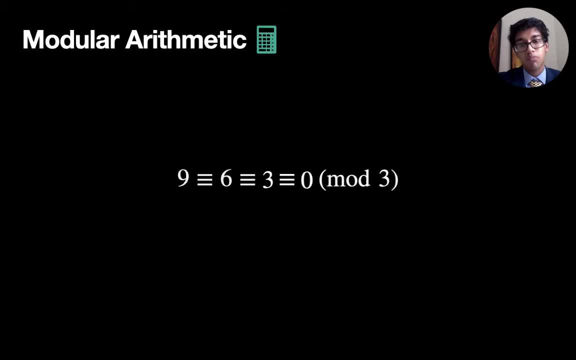 Why? It's because there are loads of other numbers that also have a remainder of zero after division by three. All of these numbers can be put in their own little group. They're all congruent to each other. Now, the next thing I want to look at is something called Freshman's Dream, which is this idea that if you have x plus y, all to the power of the prime number. 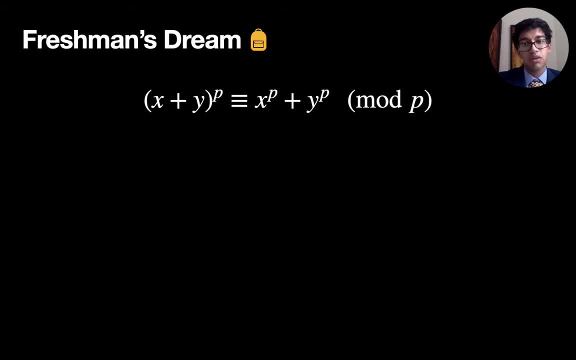 after division by the prime number, it will give you x to the p plus y to the p. The reason why it's called Freshman's Dream is because normally if you have that bracket and you expand it out, you wouldn't normally get x to the p plus y to the p. 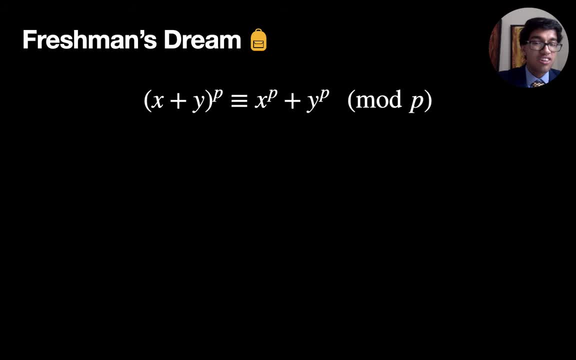 That's a rookie error, It's a freshman's error, But here it actually works. So, as an example, if you have 1 plus 2 all to the 5, p is a prime number, by the way, That's obviously 3 to the 5, 243.. 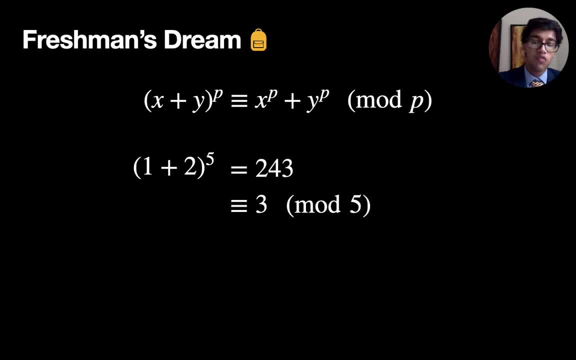 And that gives a remainder of 3 after division by 5.. Now 3 has the same remainder as 33 after division by 5.. They're all in the same equivalent group essentially, And 33 is 1 to the 5 plus 2 to the 5.. 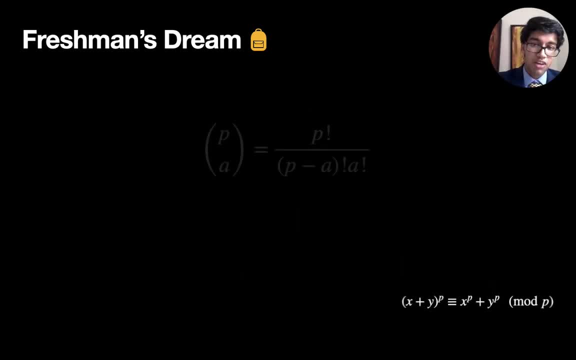 So that holds in that case, You might be wondering how we prove this. Well, it's all a-level birth mass. So imagine you have p, choose a where p is a prime number greater than a. That bit's important. We can write it as so on the right-hand side. 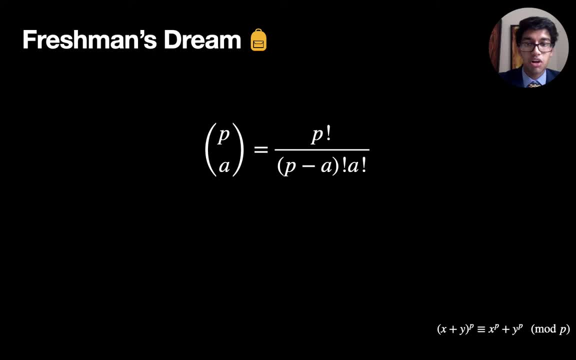 But notice that not only is p greater than p minus a and a, but p is also prime. So there are no numbers on the bottom that divide p, aka p divides p, choose a. It has a remainder of 0 after division by p. 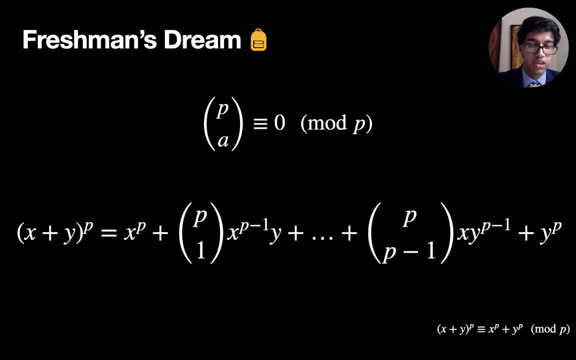 If we were just to expand out the left-hand side of our original thing, x plus y all to the p, we get the following: But notice that all the middle terms are in the form p choose a, p choose 1, p choose 2, etc. etc. 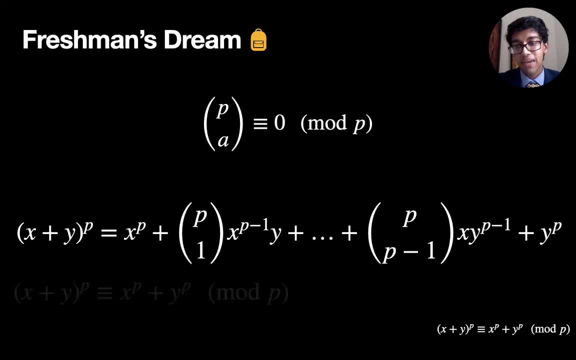 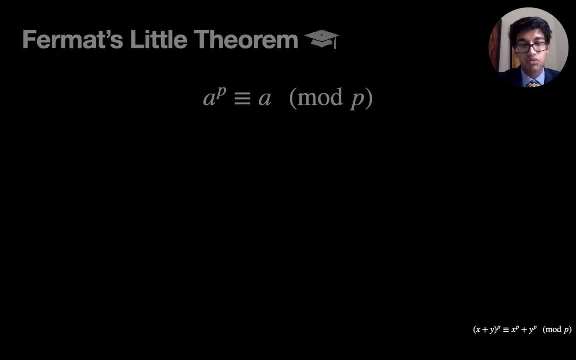 So they're all divisible by p. So the remainder, after division by p is just the first and the last term. That's how we prove freshman's dream. From this we can then derive Fermat's little theorem, so-called to distinguish it from Fermat's big. last, final deal. 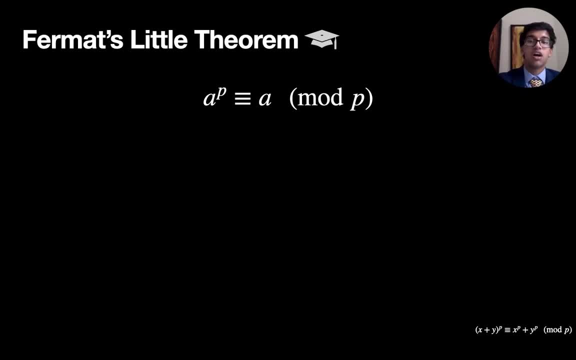 What Fermat's little theorem says is that if you have a positive integer and raise it to the power of a prime number, you'll get the original number back as the remainder after division by p. So as an example you might have 3 to 5.. 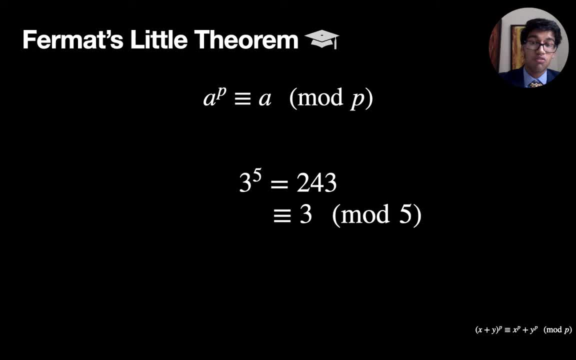 That's 243.. And that's obviously got a remainder of 3 after division by 5.. How do we prove this? Well, induction Again a level further maths. So if you have a base case when a equals 1,, 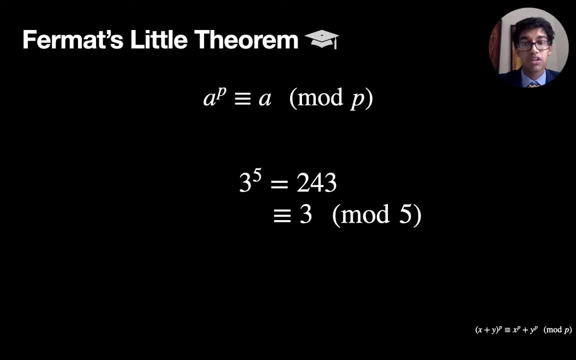 that naturally holds 1 to the p is 1.. That has a remainder of 1 after division by p. For an inductive hypothesis we assume true for a equals k And for our inductive step for k plus 1, all to the p. 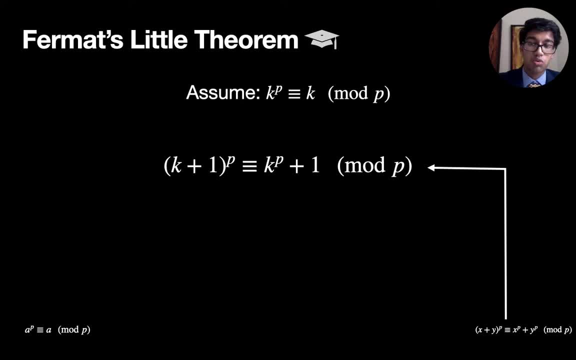 our freshman's dream tells us that k plus 1 all to the p gives a remainder of k to the p plus 1 after division by p. Our inductive hypothesis then tells us that k to the p gives a remainder of k after division by p. 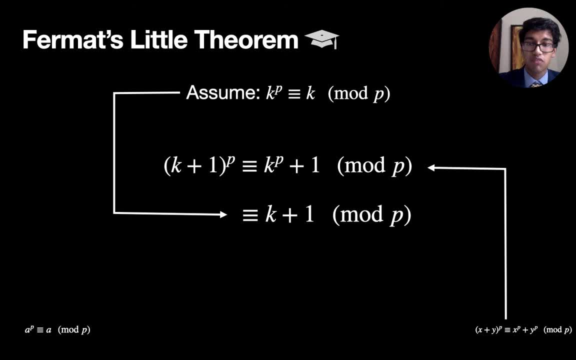 and that gives us k plus 1.. We're done. We've now shown it for k plus 1, and it's true for our base case. Therefore, this statement is true For all positive integers. Okay, enough of that for now. 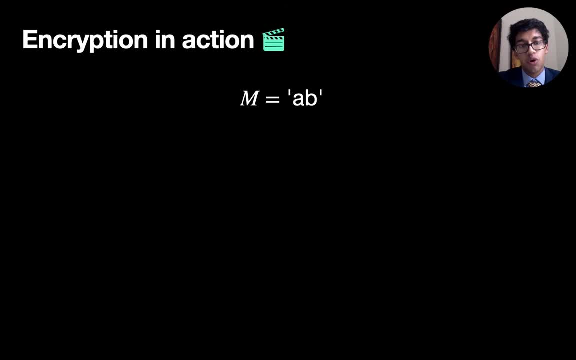 Let's see how this encryption actually works. So imagine we've got a message which is ab as an example. We need to somehow convert this into numbers, So I've said: okay, let a be equivalent to 1 and b to 2.. 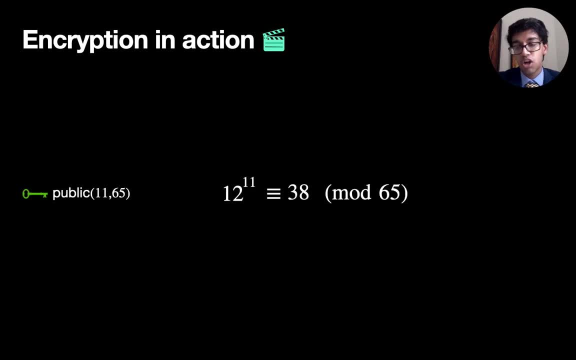 First of all, we encrypt it using our public key. So our public key provides us with two numbers. The first number is this encryption constant and our second number is this common divisor. So to find our encrypted number, we raise our message to the power of 11. 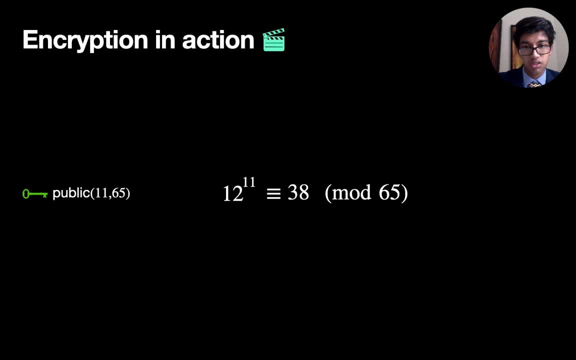 and find the remainder after division by 65. That gives us 38. That's our encrypted message. To decrypt it, we do the same thing, but with our private key. Our private key provides us with a decryption constant. So 38 to the power of 35,. 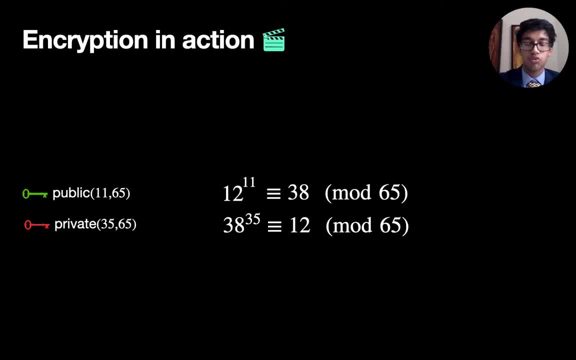 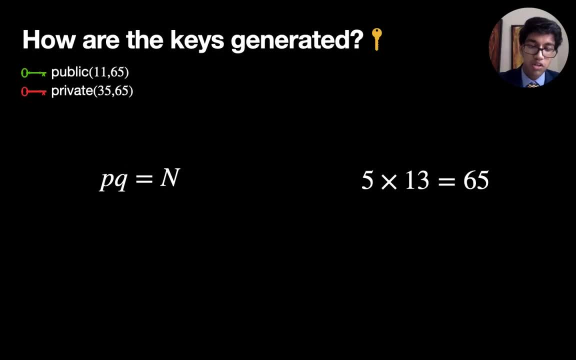 after being divided by 65, gives us a remainder of 12.. And that is our original message. You might be wondering how we actually derived these keys in the first place. Well, a common divisor is found by multiplying two prime numbers together. 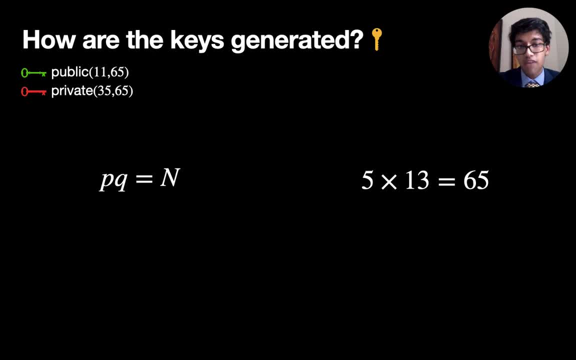 So here I've done 5 times 13,, which gives 65. In reality, these prime numbers would normally be huge. I'm talking hundreds, thousands of digits long, And so, even though multiplying them together is relatively straightforward, there's no simple, efficient way of factorising it. 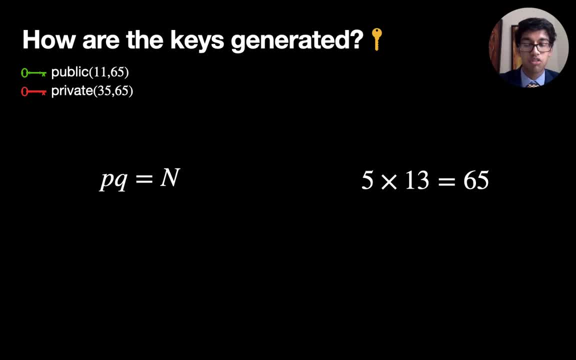 So, even though we publish n 65, to the rest of the world, it's infeasible to calculate p and q To figure out our encryption and decryption constants. we figure out the remainder two numbers that have a remainder of 1,. 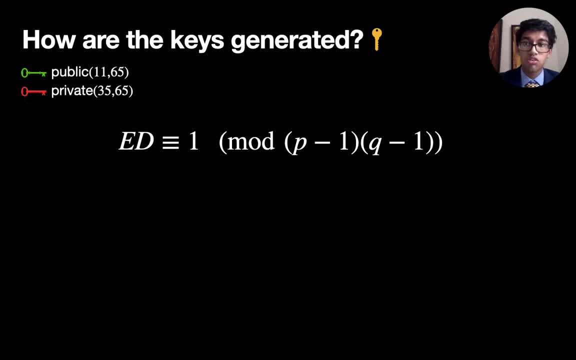 after division by p minus 1, q minus 1.. So here that shows 11 and 35.. That's 385.. And that gives a remainder of 1, after division by 48.. You might be wondering why we use this particular fact. 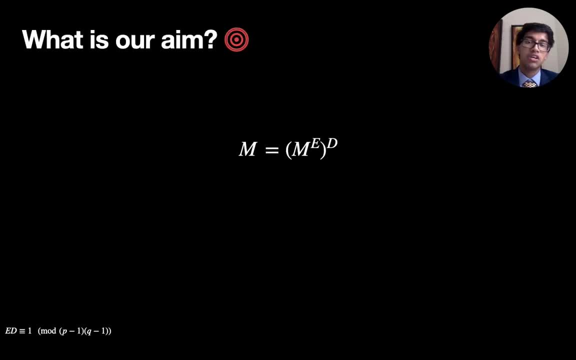 And it's all to do with our aim. Our aim here is to say, if we encrypt a message and then we decrypt it, it should lead us back to the original message. Simplifying that using simple indices rules, we get the following: 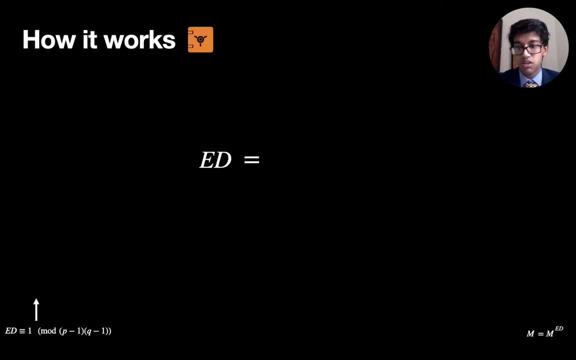 Now e d. This is where the rule comes into place. e? d is 1 plus a multiple of p minus 1, q minus 1.. So when we use this, we've got our message and we encrypt and decrypt it. 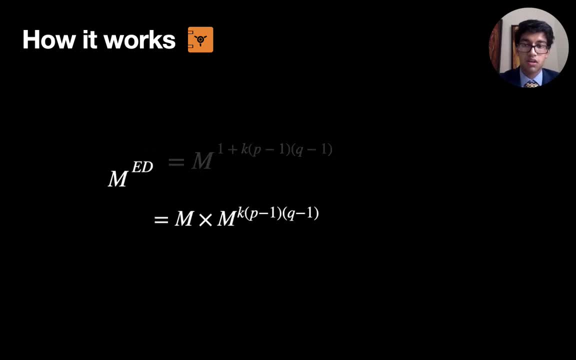 we get the following, which we can then simplify. Now, thinking back to Fermat's Little Theorem, if we have a message to the power of a prime number, that gives us our original message after division by that prime number. Note that we can change the left-hand side. 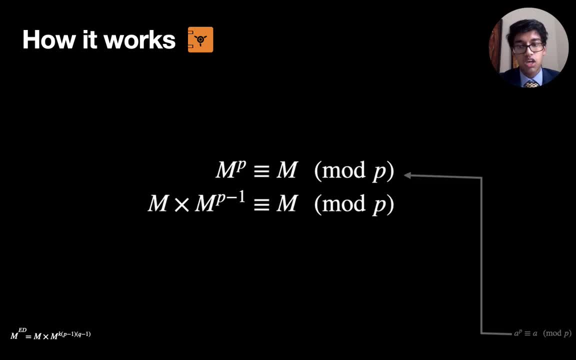 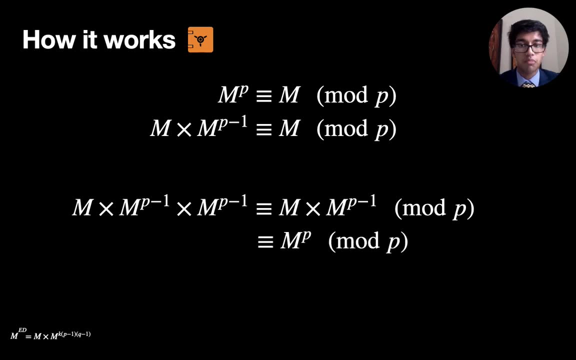 to be m times m to the p minus 1.. If we were then to multiply both left and right-hand side by m to the p minus 1, the right-hand side becomes m to the p. But we already know this has a remainder of m after division by p. 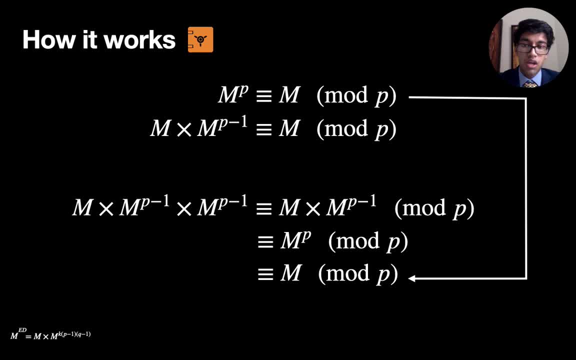 They're equivalent. They're in the same equivalence group. Now you might notice here that we can just keep repeatedly multiplying by m to the p minus 1, and we'd always get a remainder of m after division by p. So in our example of m to the e d, 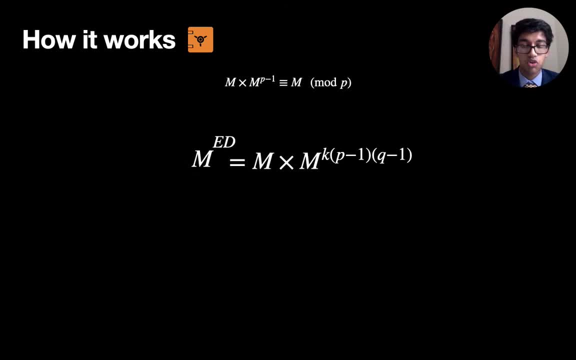 we're just multiplying by m to the p minus 1 a certain number of times, And so that just gives us a remainder of m after division by p. Now you might have noticed we're using p as our prime number, but we also had another prime number, q. 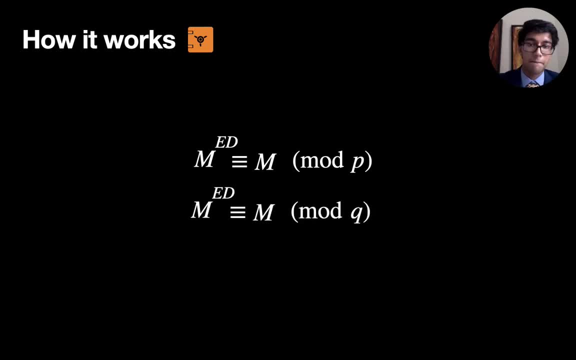 which we could have also used, and it's the same principle again. Now here you can subtract m from both sides and you'll notice that our left-hand side is divisible by both p and q, where p and q are distinct prime numbers.